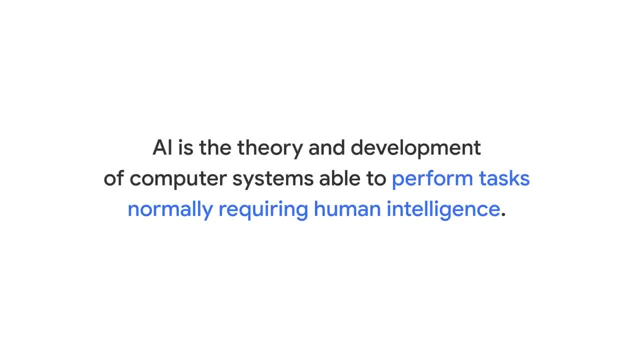 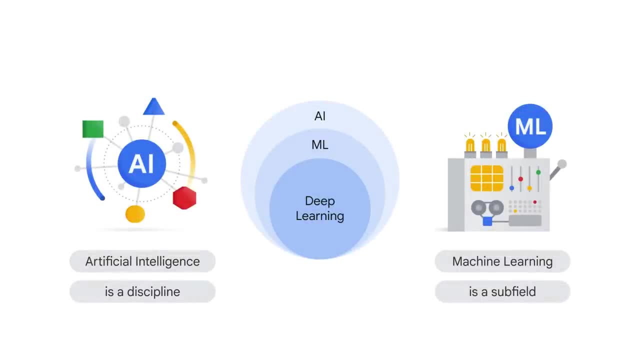 Essentially, AI has to do with the theory and methods to build machines that think and act like humans. In this discipline we have machine learning, which is a subfield of AI. It is a program or system that trains a model from input data. The trained model can make useful 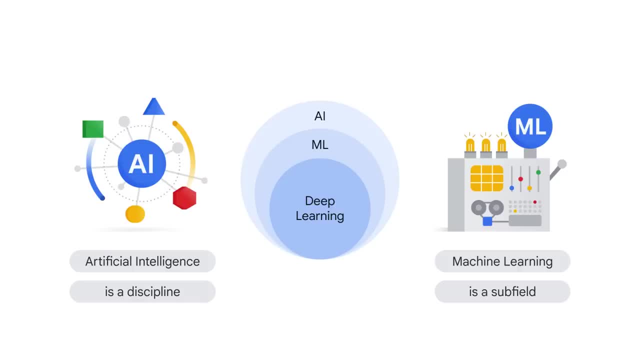 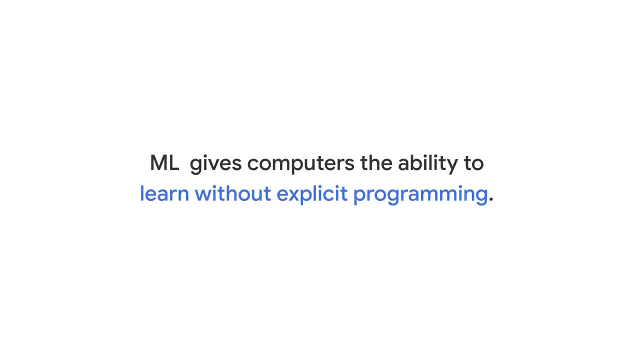 predictions from new or never-before-seen data drawn from the same one used to train the model. Machine learning gives the computer the ability to learn without explicit programming. Two of the most common classes of machine learning models are unsupervised and supervised ML models. 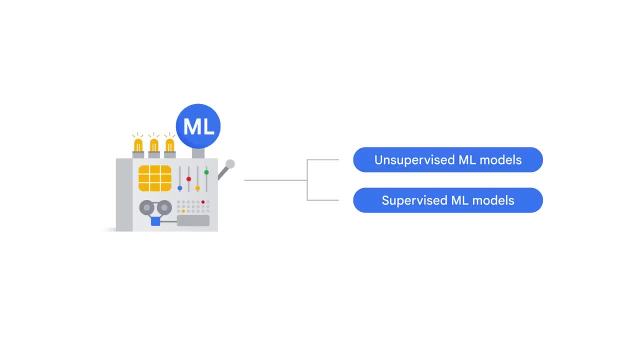 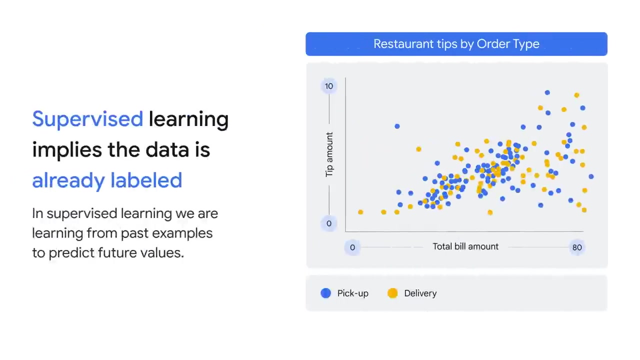 The key difference between the two is that with supervised models, we have labels. Labeled data is data that comes with a tag like a name, a type or a number. Unlabeled data is data that comes with no tag. This graph is an example of the sort of problem that a supervised 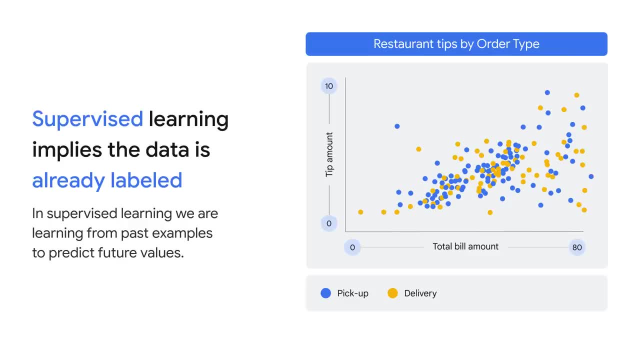 model might try to solve. For example, if a machine learning model tries to solve a problem with a tag, it will be able to do this. For example, let's say you are the owner of a restaurant. You have historical data of the bill amount and how much different people tipped, based on order. 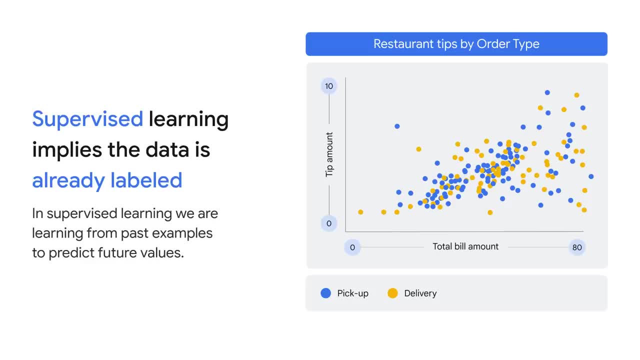 type, whether it was picked up or delivered. In supervised learning, the model learns from past examples to predict future values, in this case tips. So here the model uses the total bill amount to predict the future tip amount, based on whether an order was picked up or delivered. 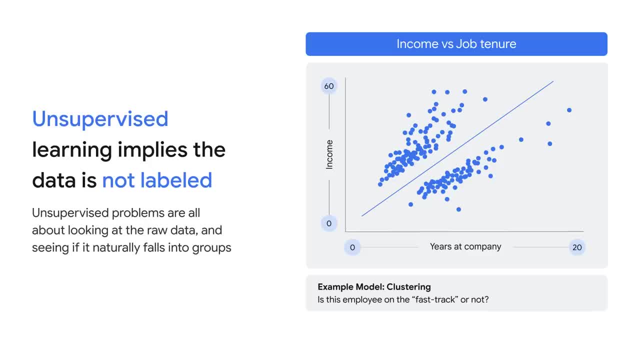 This is an example of the sort of problem that an unsupervised model might try to solve. So here you want to look at tenure and income and then group or cluster employees to see whether someone is on the fast track. Unsupervised problems are all about. 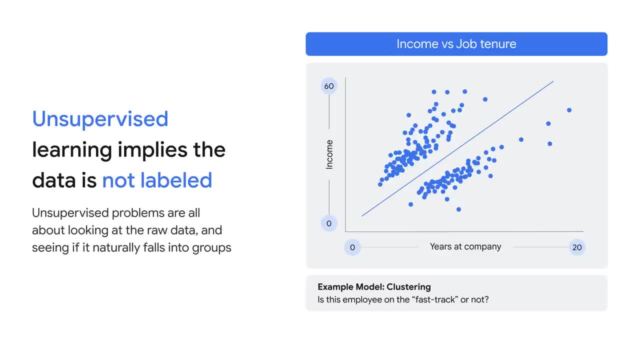 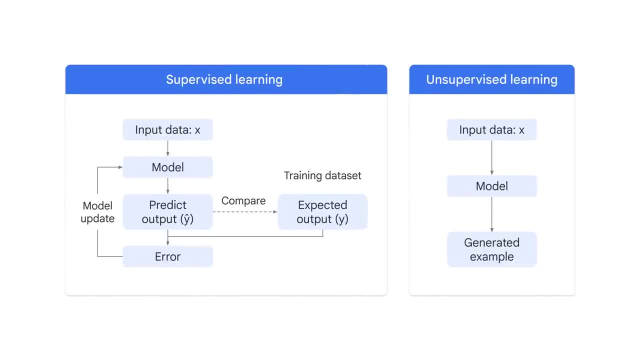 discovery about looking at the raw data and seeing if it naturally falls into groups. Let's get a little deeper and show this graphically as understanding the model. These concepts are the foundation for your understanding of generative AI In supervised learning testing. data values or X are input into the model. The model outputs: 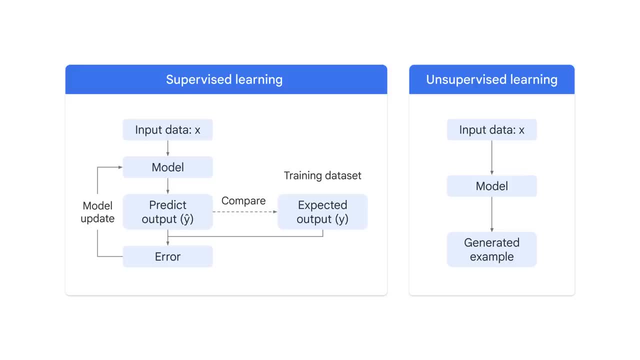 a prediction and compares that prediction to the training data used to train the model. If the predicted test data values and actual training data values are far apart, that's called error And the model tries to reduce the training data values. and the model tries to reduce the. 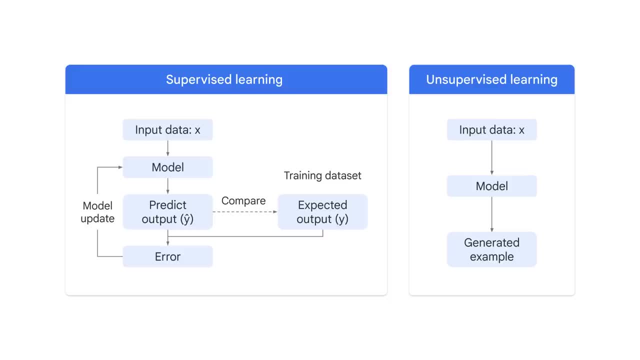 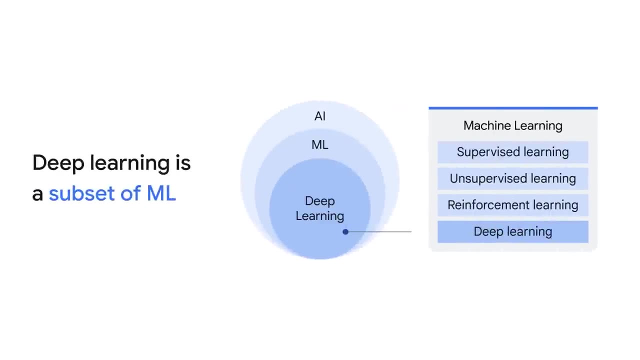 error. A model is able to reduce this error until the predicted and actual values are closer together. This is a classic optimization problem. Now that we've explored the difference between artificial intelligence and machine learning, and supervised and unsupervised learning, let's briefly explore where deep learning fits as a subset of machine learning methods. 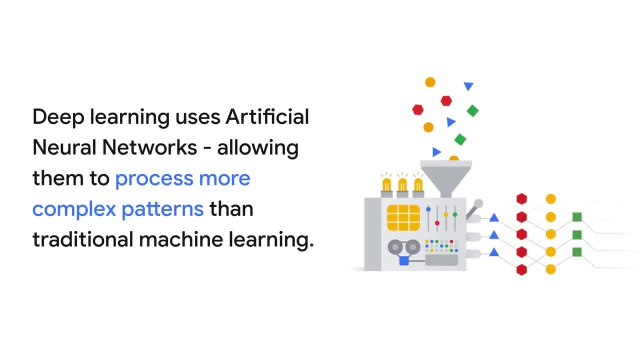 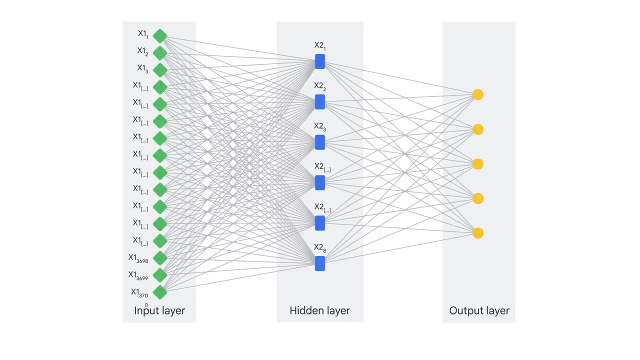 While machine learning is a broad field that encompasses many different techniques, type of machine learning that uses artificial neural networks, allowing them to process more complex patterns than machine learning. Artificial neural networks are inspired by the human brain. They are made up of many interconnected nodes or neurons that can learn to perform tasks. 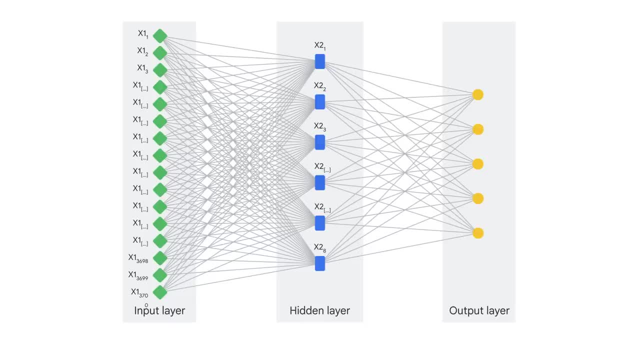 by processing data and making predictions. Deep learning models typically have many layers of neurons, which allows them to learn more complex patterns than traditional machine learning models, And neural networks can use both labeled and unlabeled data. This is called semi-supervised learning. 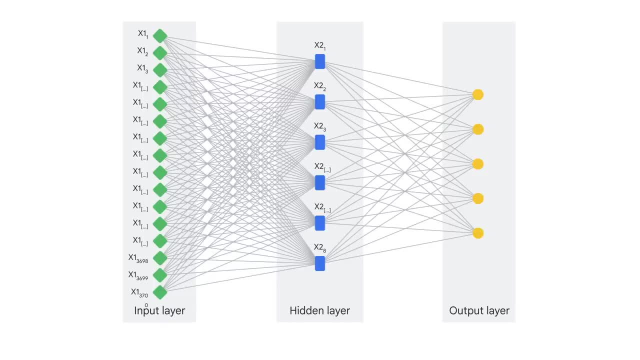 In semi-supervised learning, a neural network is trained on a small amount of labeled data and a large amount of unlabeled data. The labeled data helps the neural network to learn the basic concepts of the task, while the unlabeled data helps the neural network to generalize to new examples. 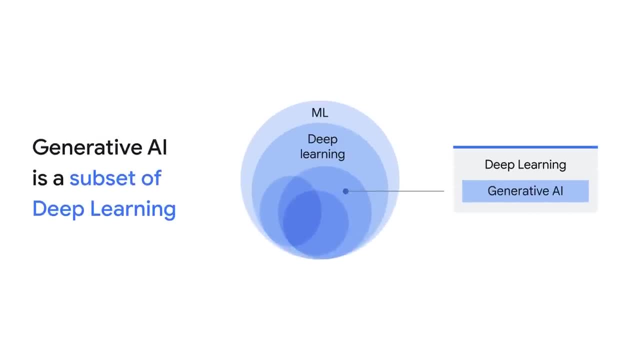 Now we've finally got to where generative AI fits into this AI discipline. Gen AI is a subset of deep learning, which means it uses artificial neural networks, can process both labeled and unlabeled data, using supervised, unsupervised and semi-supervised. 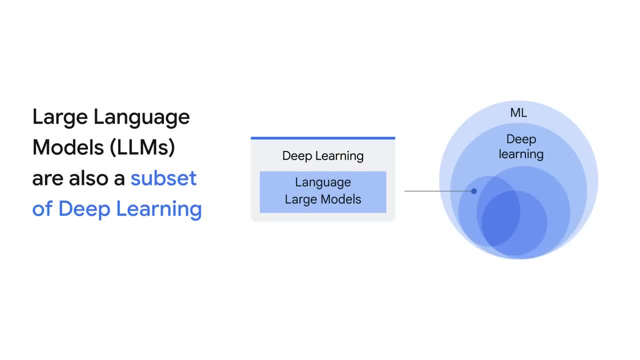 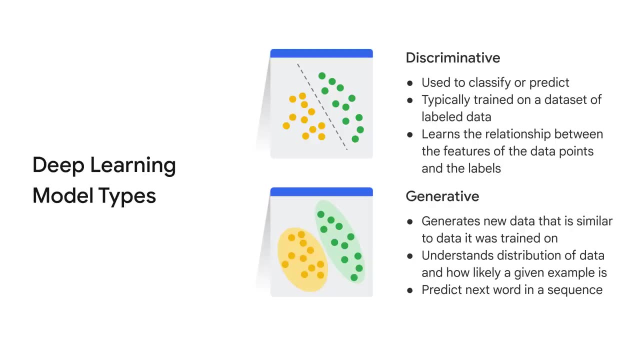 methods. Large language models are also a subset of deep learning or machine learning. models in general can be divided into two types: generative and discriminative. A discriminative model is a type of model that is used to classify or predict labels for data points. 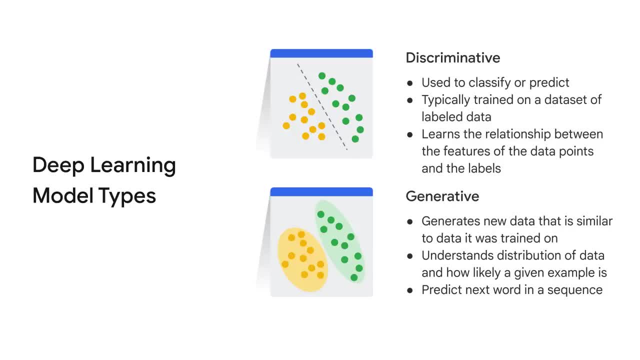 Discriminative models are typically trained on a data set of labeled data points and they learn the relationship between the features of the data points and the labels. Once a discriminative model is trained, it can be used to predict the label for new data points. 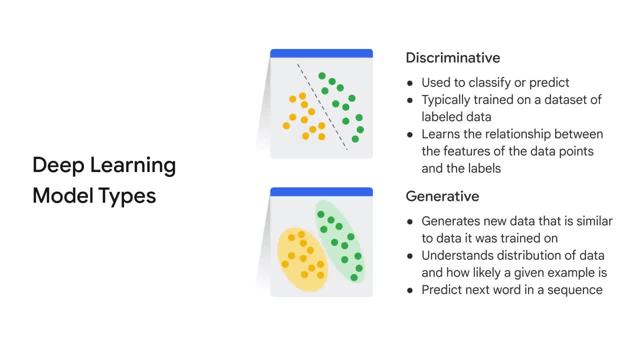 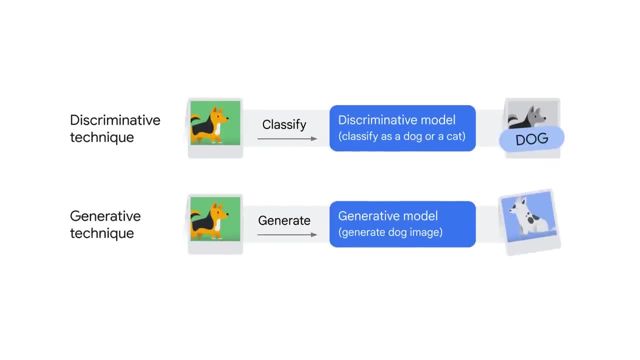 A generative model generates new data instances based on a learned probability distribution of existing data. Thus, models generate new content. Take this example: Here the discriminative model learns the conditional probability distribution, or the probability of y- our output- given x- our input, that this is a dog and classifies it as a dog and not a cat. 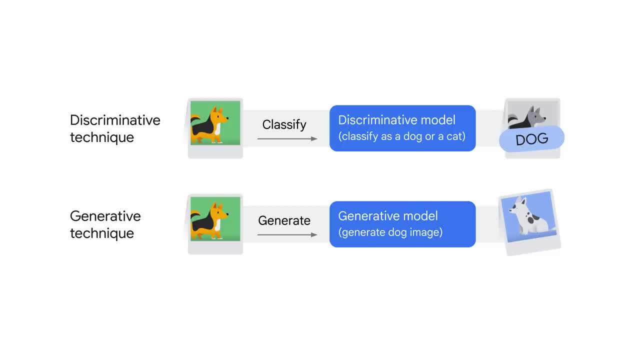 The generative model learns the joint probability distribution or the probability of x and y, and predicts the conditional probability that this is a dog, and can then generate a picture of a dog. So, to summarize, generative models can generate new data instances. 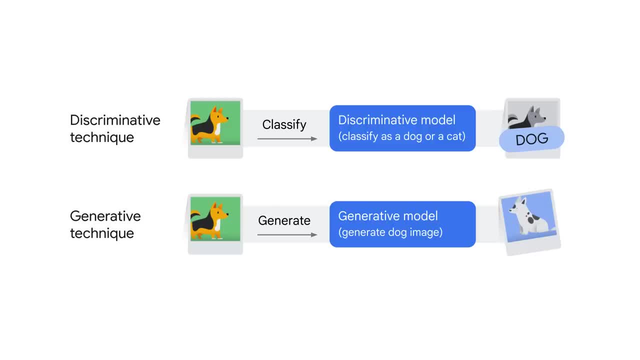 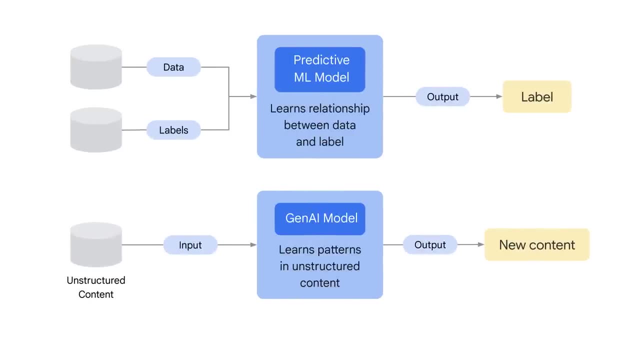 while discriminative models discriminate between different kinds of data instances. The top image shows a traditional machine learning model which attempts to learn the relationship between the data and the label, or what you want to predict. The bottom image shows a generative AI model which attempts to learn patterns on content. 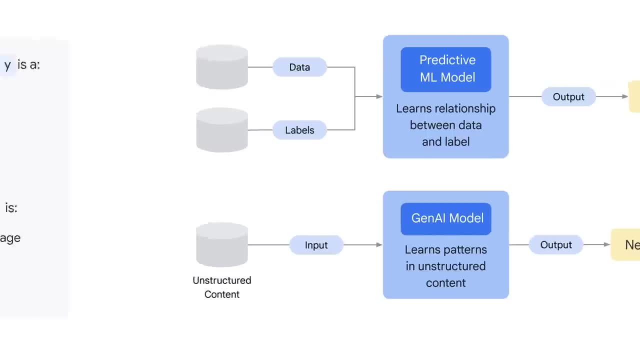 so that it can generate new content. A good way to distinguish what is GenAI what is not is showing three machinery, An yourself as well as the behavior of the онself. a better way to distinguish what is GenAI and what is not. 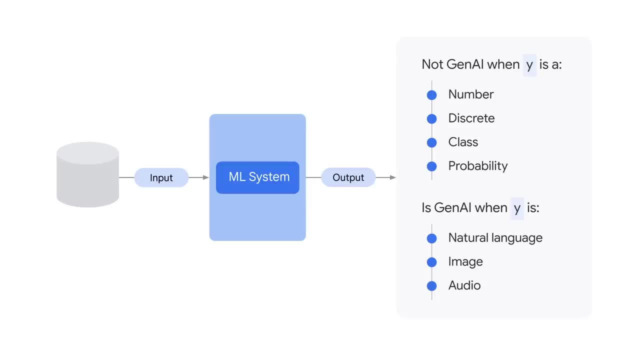 in this illustration. It is not Gen AI when the output or Y or label is a number or a class of, for example, spam or not spam, or a probability. It is Gen AI when the output is natural language, like speech or text, an image or audio, for example. Visualizing this mathematically would 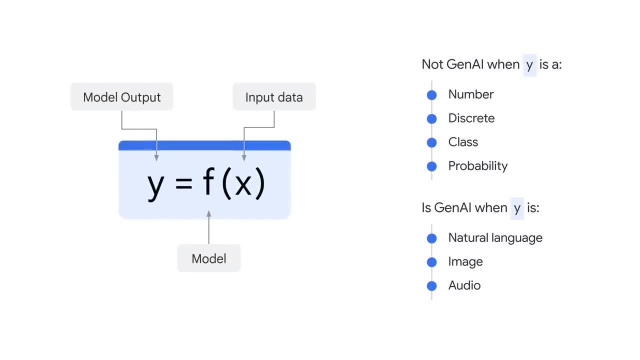 look like this, If you haven't seen this for a while: the Y is equal to F of X equation calculates the dependent output of a process given different inputs. The Y stands for the model output, The F embodies the function used in the calculation and the X represents the input or inputs used for the. 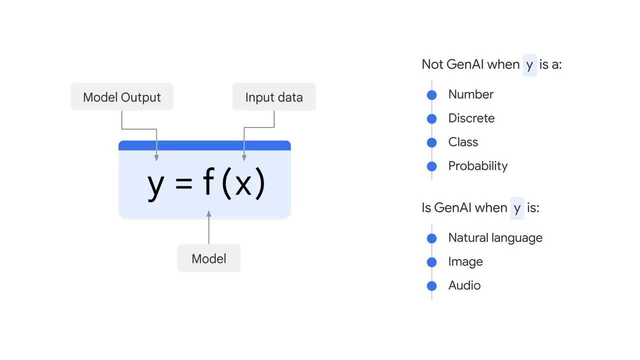 formula. So the model output is a function of all the inputs. If the Y is a number, like predicted sales, it is not Gen AI. If Y is a sentence like defined sales, it is generative, as the question would elicit a text response. The response would be based on all the massive, large data, the model. 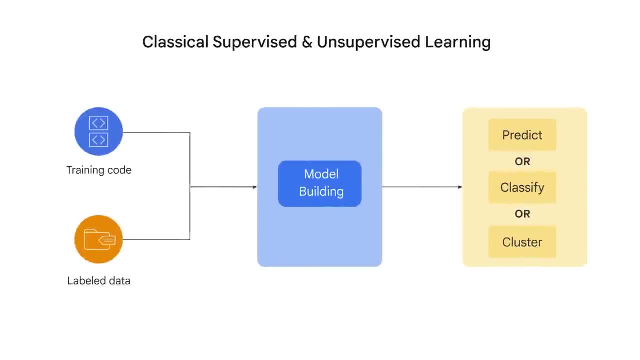 was already trained on. To summarize at a high level: the traditional classical, supervised and unsupervised learning process takes training, code and label data to build a model. Depending on the model, the model is a model. If the model is a number, like predicted sales, it is not Gen AI. 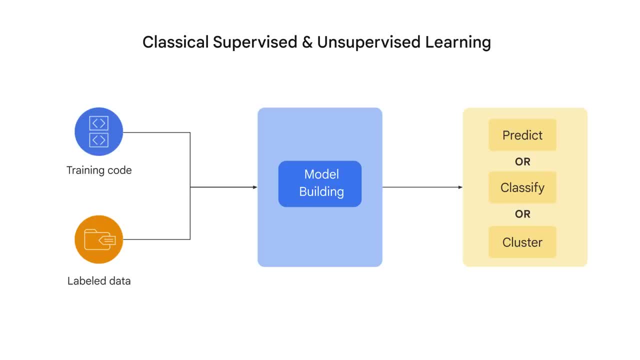 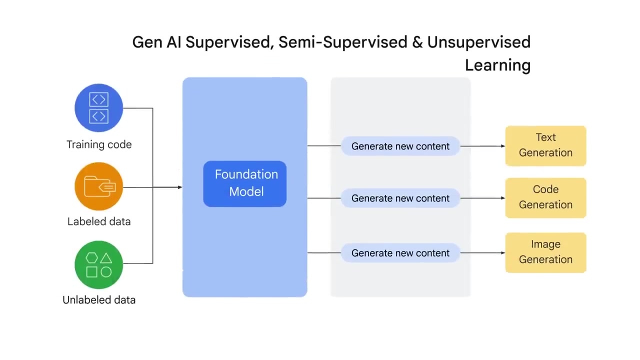 The model can give you a prediction. It can classify something or cluster something. We use this example to show you how much more robust the Gen AI process is. The Gen AI process can take training, code, label data and unlabel data of all data types and build a foundation model. 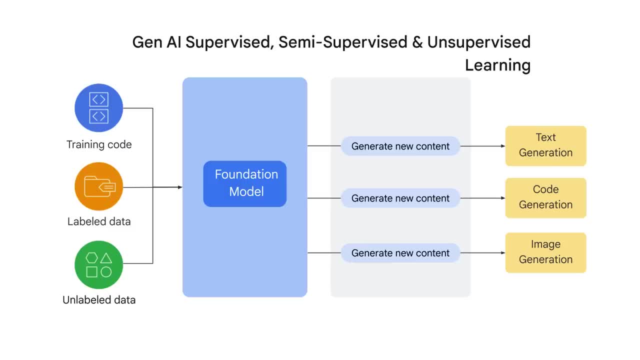 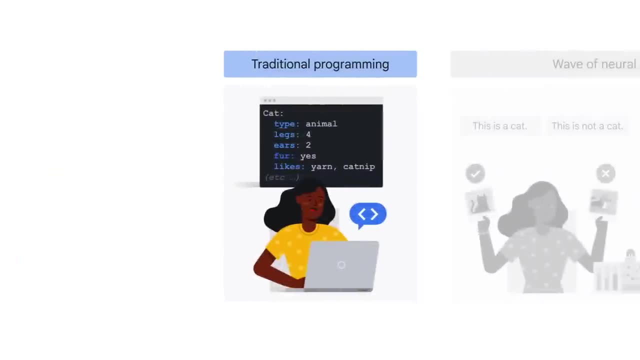 The foundation model can then generate new content, For example text code, images, audio video etc. We've come a long way, from traditional programming to neural networks, to generative models. In traditional programming we used to have to hard code the rules for distinguishing a cat. 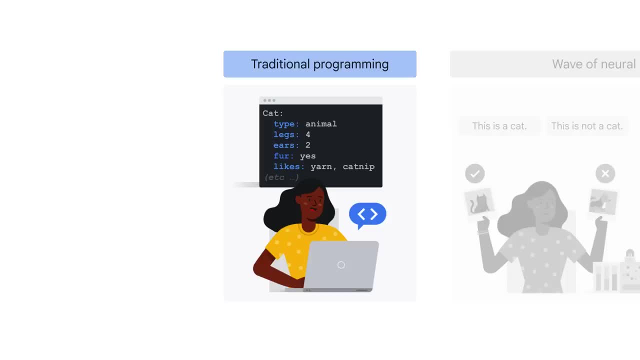 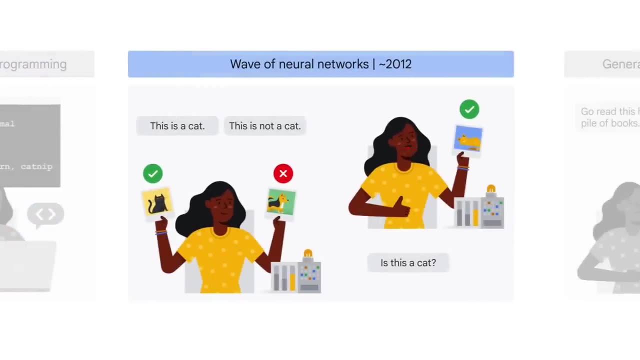 The type: animal Legs, fur Ears, two Fur- yes, Likes yarn and catnip In the wave of neural networks we could give the network pictures of cats and dogs and ask: is this a cat? And 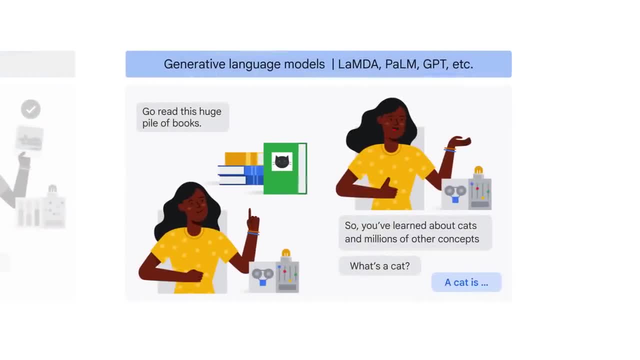 it would predict a cat In the generative wave. we as users can generate our own content, Whether it be text, images, audio video, etc. For example, models like Palm or Pathways Language Model or Lambda Language Model for Dialog Applications, and just very, very large data from 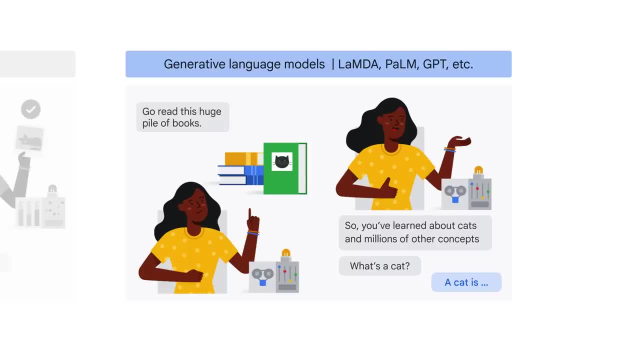 the multiple sources across the internet and build foundation language models we can use simply by asking a question, Whether typing it into a prompt or verbally talking, into the prompt itself. So when you ask it what's a cat, It can give you everything it has learned about a cat. 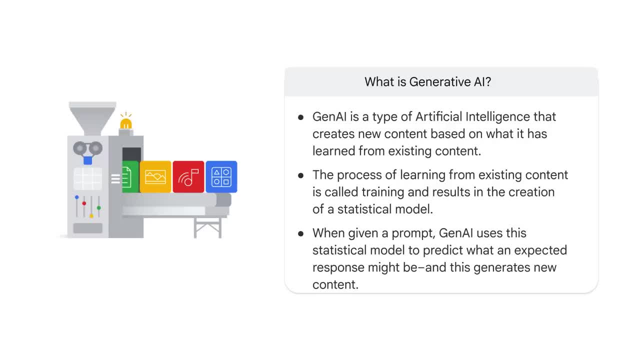 Now we come to our formal definition. What is generative AI? Gen AI is a type of artificial intelligence that creates new content based on what it has learned from existing content. The process of learning from existing content is called training and results in the creation of a statistical model. When given a prompt, Gen AI uses the model to predict what an expected. 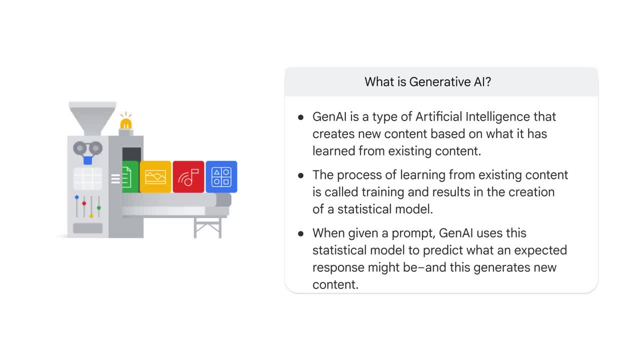 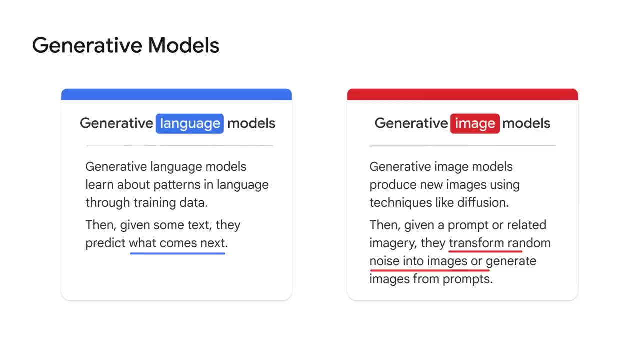 response might be, and this generates new content. Essentially, it learns the underlying structure of the data and can then generate new samples that are similar to the data it was trained on. As previously mentioned, a generative language model can take what it has learned from the examples it's been shown and 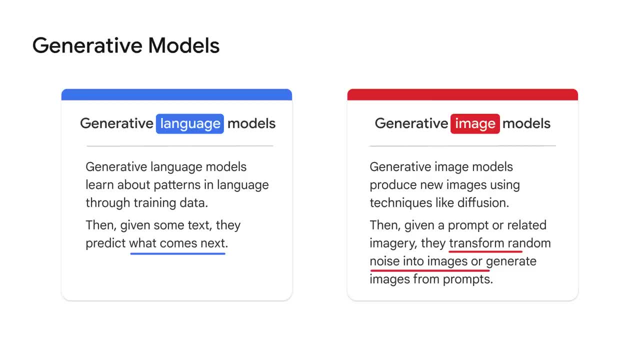 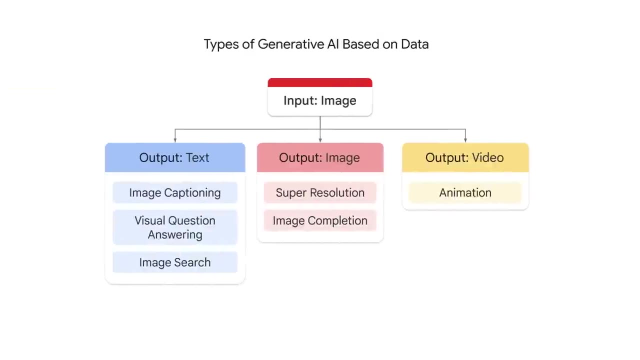 creates something entirely new based on that information. Large language models are one type of generative AI, since they generate novel combinations of text in the form of natural-sounding language. A generative image model takes an image as input and can output text, another image or video. For example, under the output text you can get visual question answering or 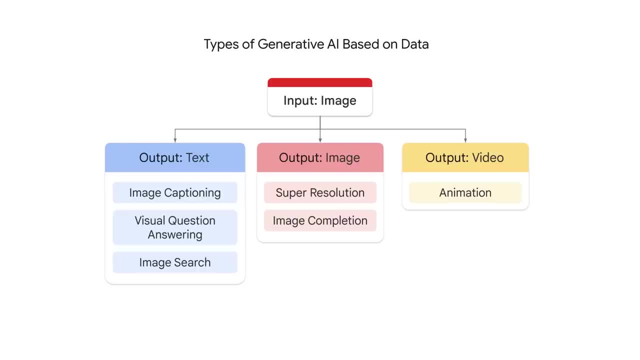 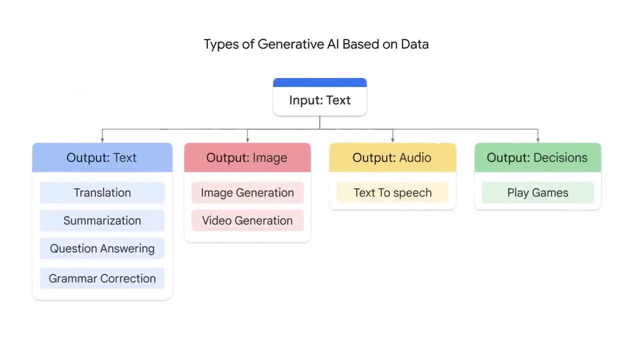 While under output image an image completion is generated And under output video animation is generated, A generative language model takes text as input and can output more text, an image, audio or decisions, For example, under the output text. 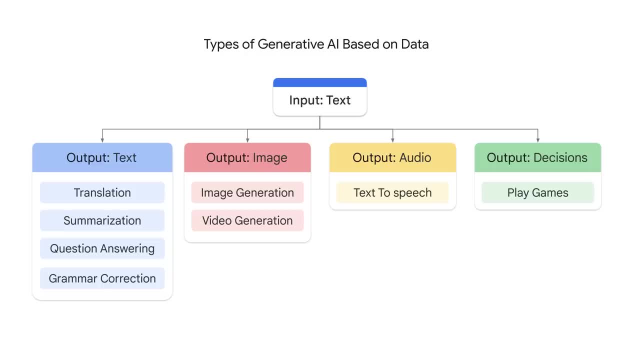 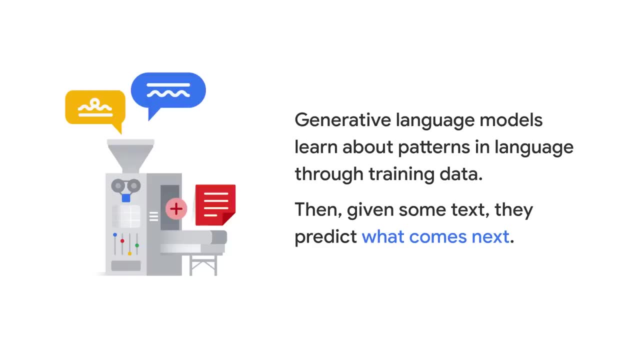 question answering is generated And under output image, a video is generated. We've stated that generative language models learn about patterns in language through training data. Then, given some text, they predict what comes next. Thus, generative language models are pattern matching systems. 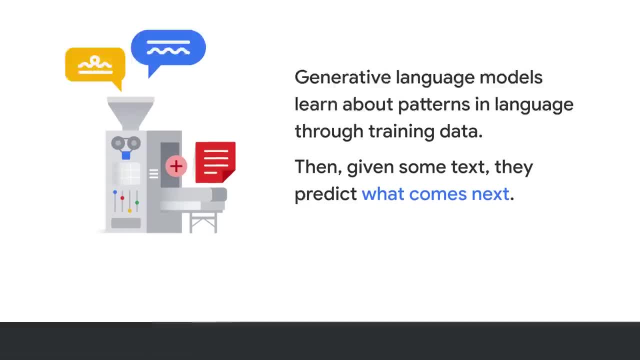 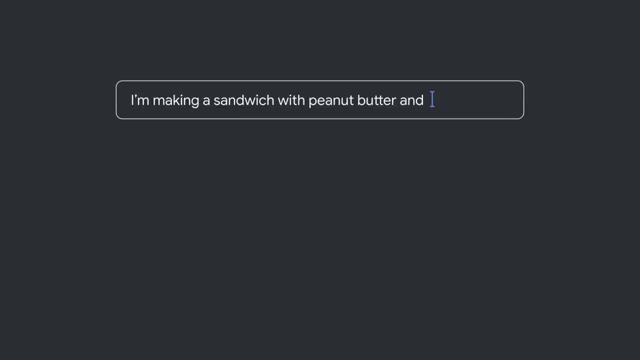 They learn about patterns based on the data you provide. Here is an example Based on things it's learned from its training data. it offers predictions of how to complete this sentence. I'm making a sandwich with peanut butter and jelly. Here is the same example using BARD. 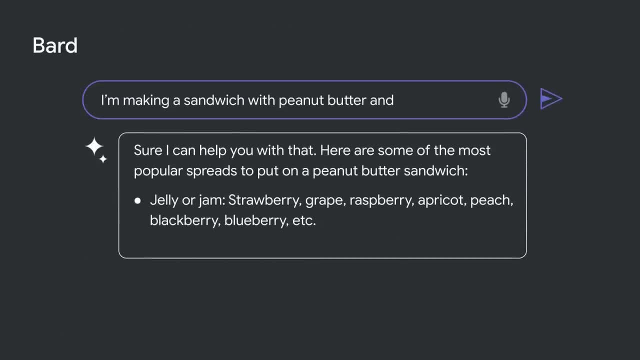 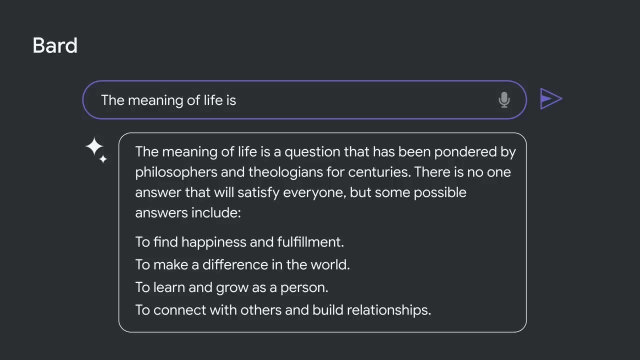 which is trained on a massive amount of text data and is able to communicate and generate human-like text in response to a wide range of prompts and questions. Here is another example: The meaning of life is, and BARD gives you a contextual answer and then shows the highest probability response. 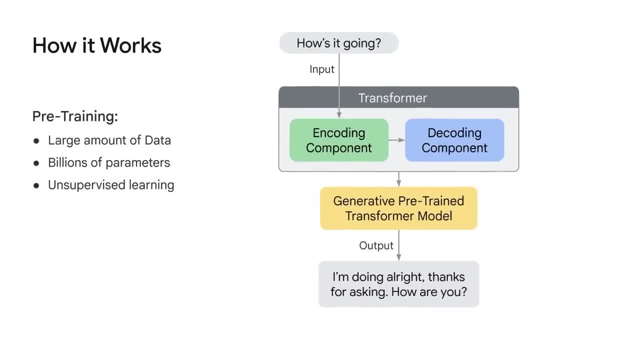 The power of generative AI comes from the use of transformers. Transformers produced the 2018 revolution in natural language processing At a high level. a transformer model consists of an encoder and decoder. The encoder encodes the input sequence and passes it to the decoder, which learns how to decode the representation. 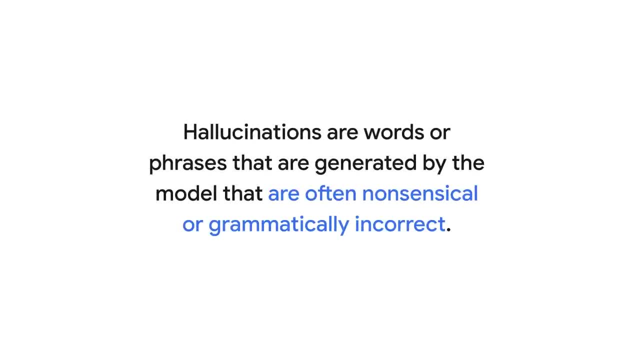 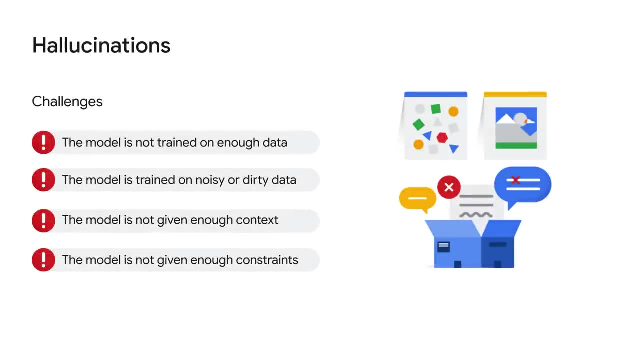 for a relevant task In transformers. hallucinations are words or phrases that are generated by the model, that are often nonsensical or grammatically incorrect. Hallucinations can be caused by a number of factors, including the model is not trained on enough data. 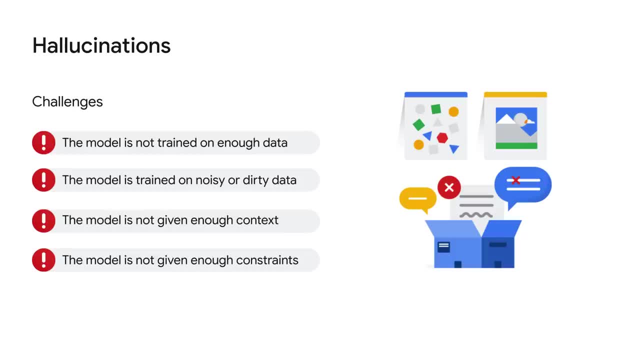 or the model is trained on noisy or dirty data, or the model is not given enough context, or the model is not given enough constraints. Hallucinations can be a problem for transformers because they can make the output text difficult to understand. they can also make the model more likely to generate. 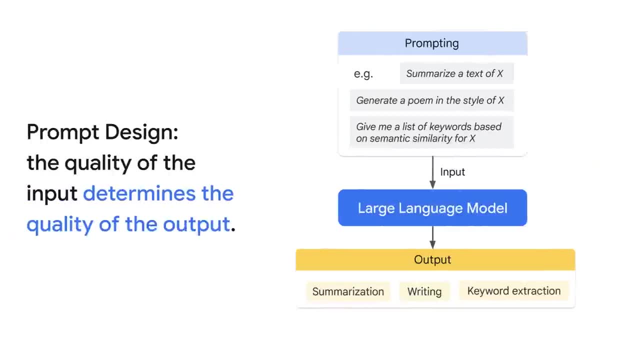 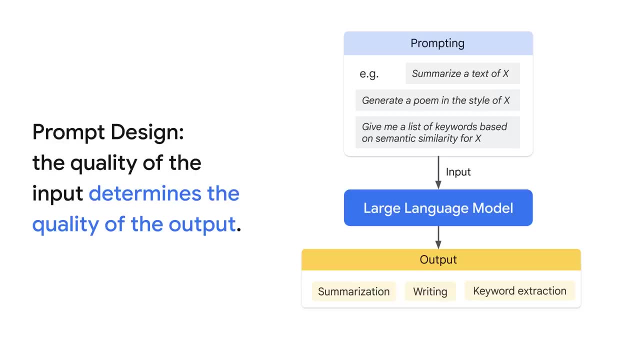 incorrect or misleading information. A prompt is a short piece of text that is given to the large language model as input, and it can be used to control the output of the model in a variety of ways. Prompt disarming is the process of creating a prompt. 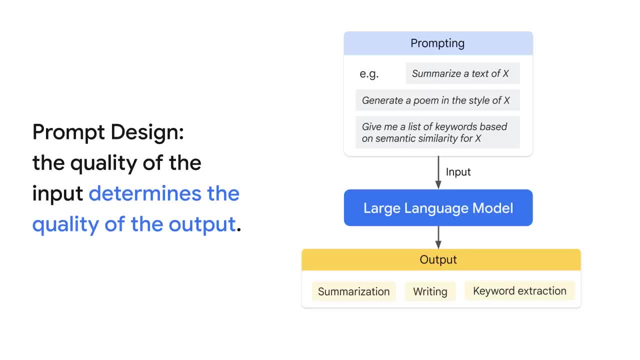 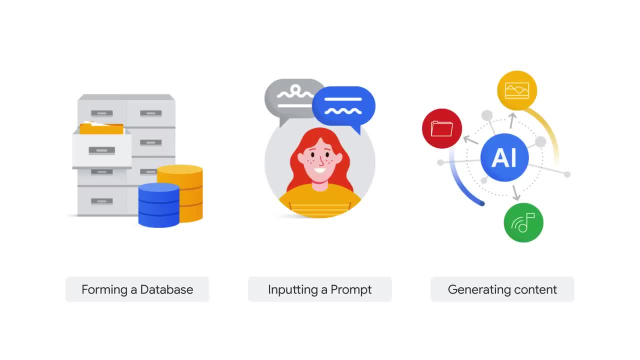 that will generate the desired output from a large language model. As previously mentioned, GenAI depends a lot on the training data that you have fed into it, and it analyzes the patterns and structures of the input data and thus learns, But with access to a browser-based prompt. 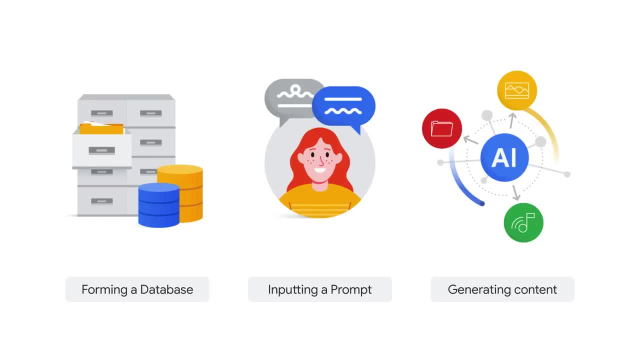 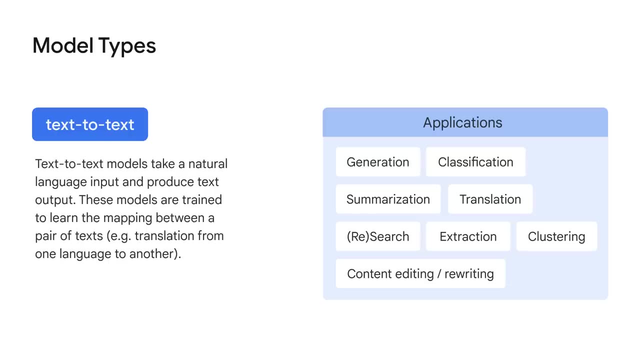 you, the user, can generate your own content. We've shown illustrations of the types of input based upon data. Here are the associated model types: text-to-text. Text-to-text models take a natural natural language input and produces a text output. 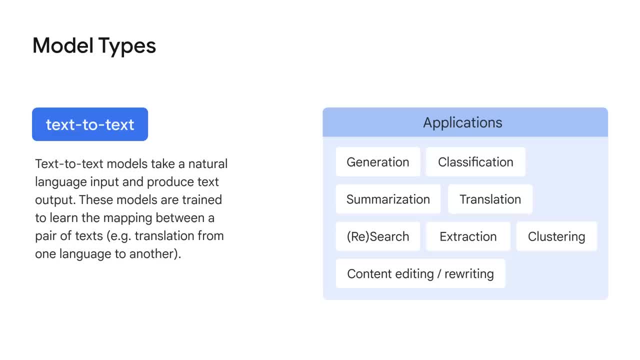 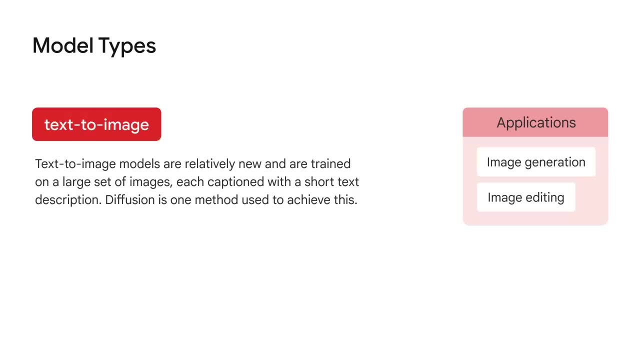 These models are trained to learn the mapping between a pair of texts, eg, for example, translation from one language to another. Text-to-image. Text-to-image models are trained on a large set of images, each captioned with a short text description. 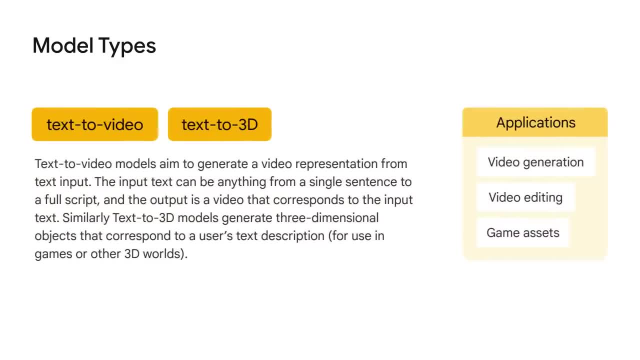 Diffusion is one method used to achieve this. Text-to-video and text-to-3D Text-to-video models aim to generate a video representation, but they are also trained to learn the mapping between a pair of texts, eg, for example, translation from text input. 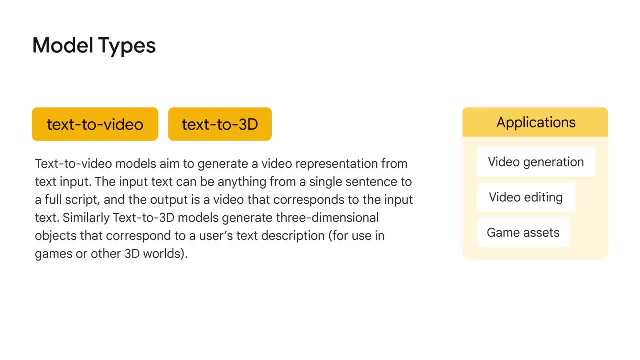 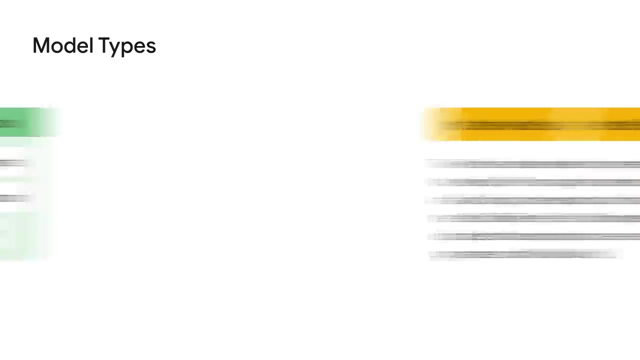 The input text can be anything from a single sentence to a full script, and the output is a video that corresponds to the input text. Similarly, text-to-3D models generate three-dimensional objects that correspond to a user's text description, For example. this can be used in games or other 3D worlds. 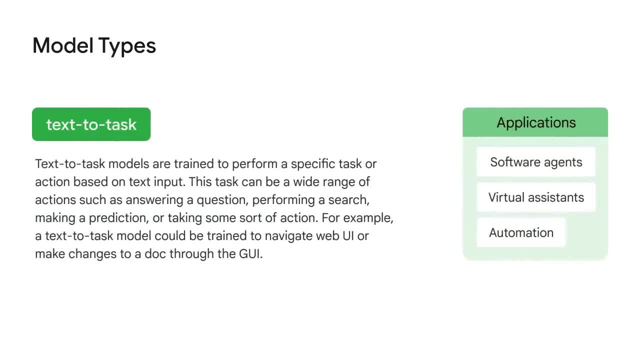 Text-to-task. Text-to-task. Text-to-task models are trained to perform a defined task or action based on text input. This task can be a wide range of actions, such as answering a question, performing a search, making a prediction or taking some sort of action. 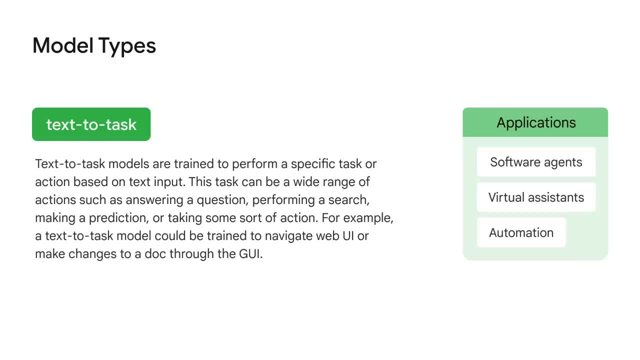 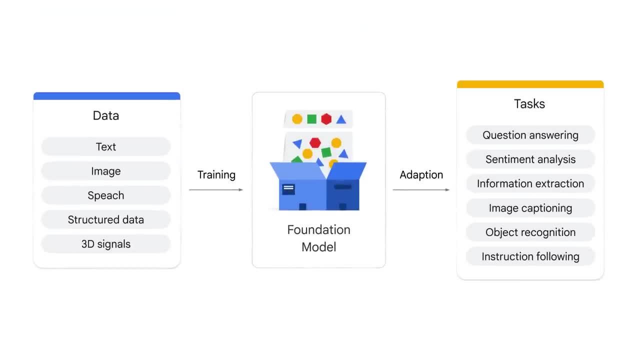 For example, a text-to-task model could be trained to navigate a web UI or make changes to a doc through the GUI. A foundation model. A foundation model is a large AI model pre-trained on a vast quantity of data designed to be adapted or fine-tuned. 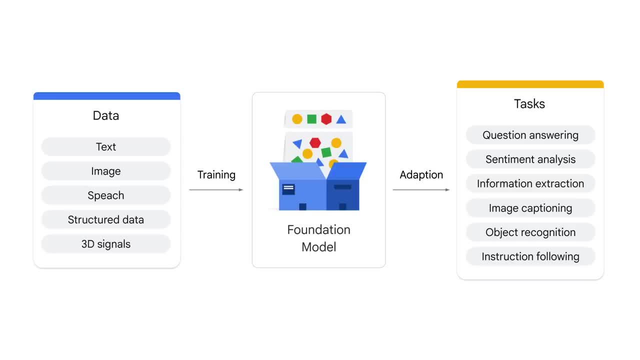 to a wide range of downstream tasks, such as sentiment analysis, image captioning and object recognition. Foundation models have the potential to revolutionize many industries, including healthcare, finance and customer service. They can be used to detect fraud and provide personalized customer support. 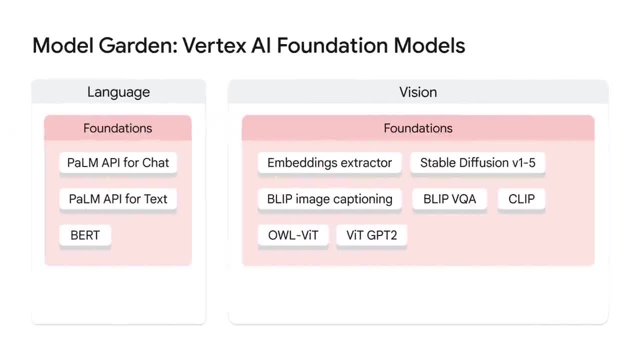 Vertix AI offers a model garden that includes foundation models. The language foundation models include Palm API for chat and text. The vision foundation models includes stable diffusion, which has been shown to be effective at generating high-quality images from text descriptions. Let's say: you have a use case. 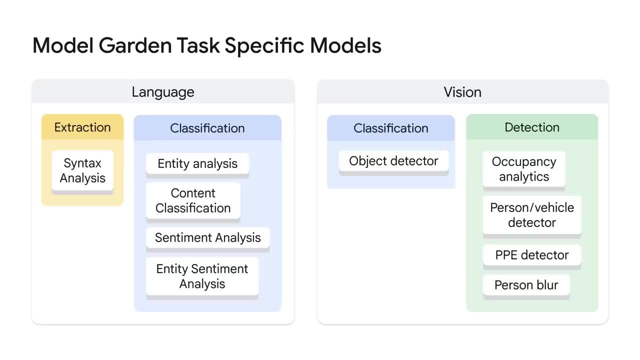 where you need to gather sentiments about how your customers are going to respond to your questions. You can use the classification task sentiment analysis task model for just that purpose. And what if you needed to perform occupancy analytics? There is a task model for your use case. 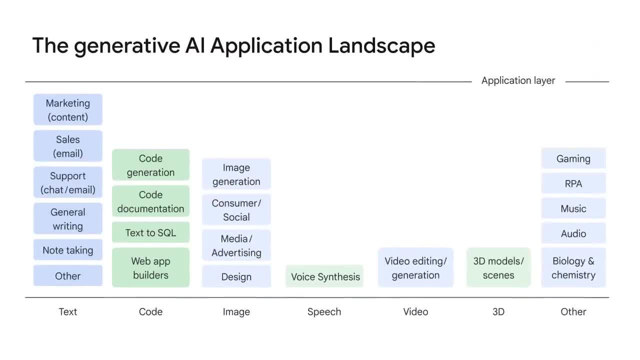 Shown here are Gen AI applications. Let's look at an example of code generation shown in the second block under code at the top, And this is a test model for code generation. And this is a test model for code generation In this example. 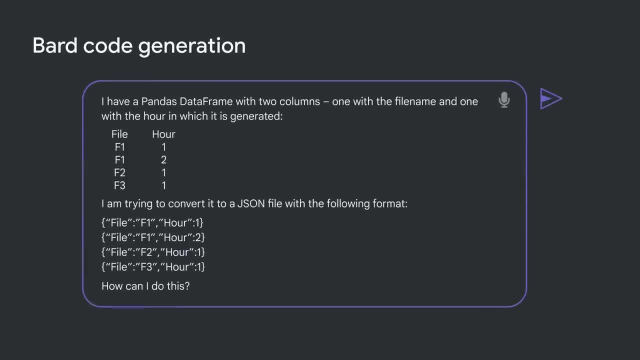 I've input a code file conversion problem Converting from Python to JSON. I use BART and I insert into the prompt box the following: I have a pandas data frame with two columns, one with the file name and one with the hour in which it is generated. 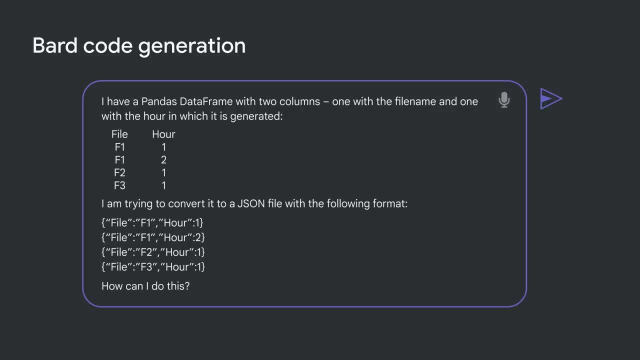 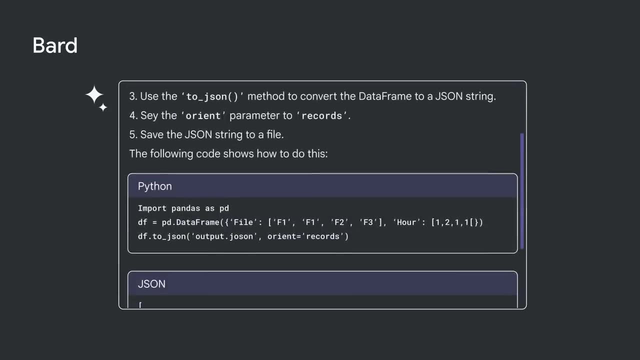 I'm trying to convert this into a JSON file in the format shown on screen. BART returns the steps I need to do this. BART returns the steps I need to do this. BART returns the steps I need to do this And the code snippet. 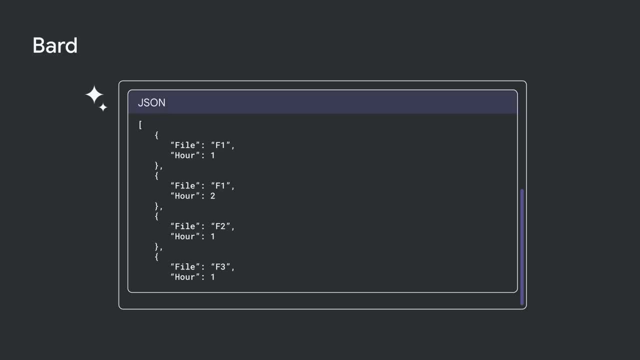 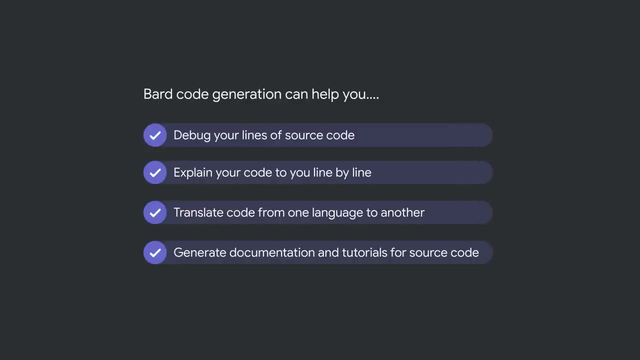 And here my output is in a JSON format. It gets better. I happen to be using Google's free browser-based Jupyter Notebook, known as Colab, and I simply export the Python code to Google's Colab. To summarize: BART code generation can help you. 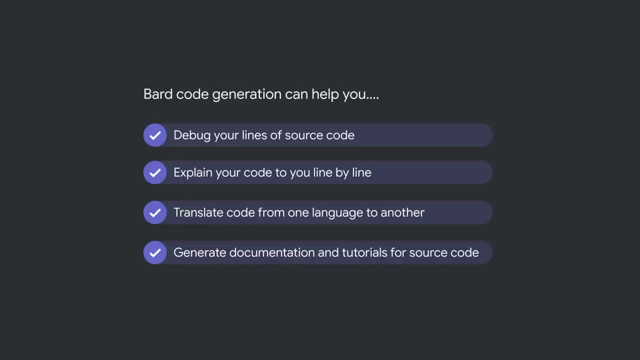 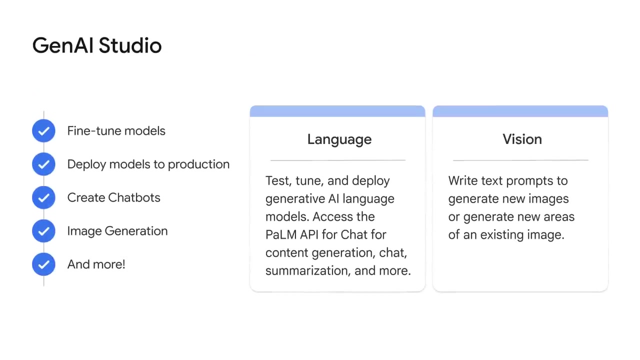 debug your lines of source code, explain your code to you line by line, craft SQL queries for your JSON code, create a database for your database, translate code from one language to another and generate documentation and tutorials for source code. Generative AI Studio lets you quickly explore. 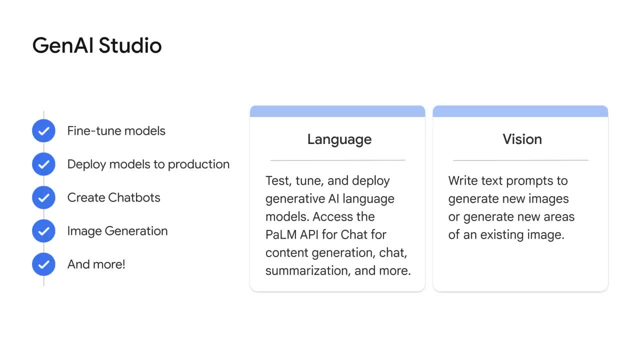 and customize Gen AI models that you can leverage in your applications on Google Cloud. Generative AI Studio helps developers create and deploy Gen AI models by providing a variety of tools and resources that make it easy to use. For example, there's a library of pre-trained models. 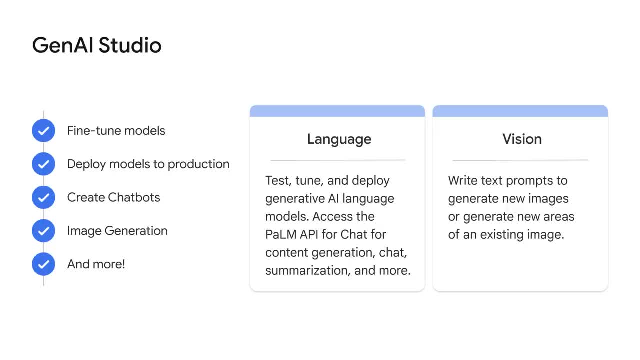 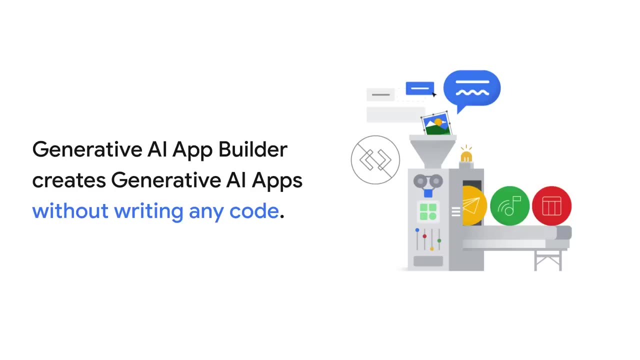 There is a tool for fine-tuning models, There is a tool for deploying models to production And there is a community forum for developers to share ideas and collaborate. Generative AI App Builder lets you create Gen AI apps without having to write any code.